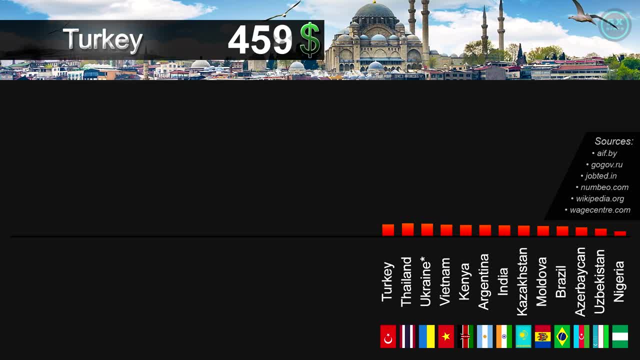 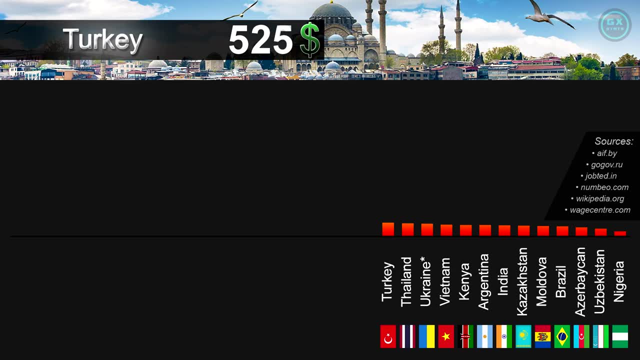 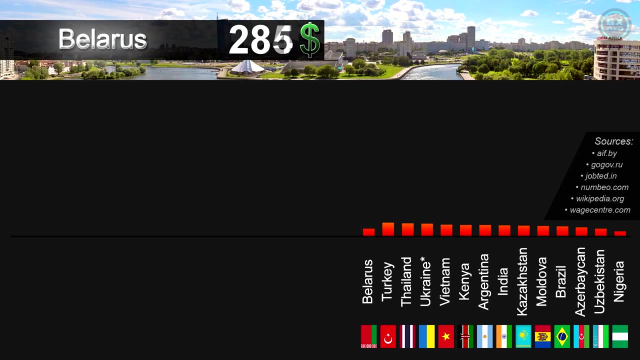 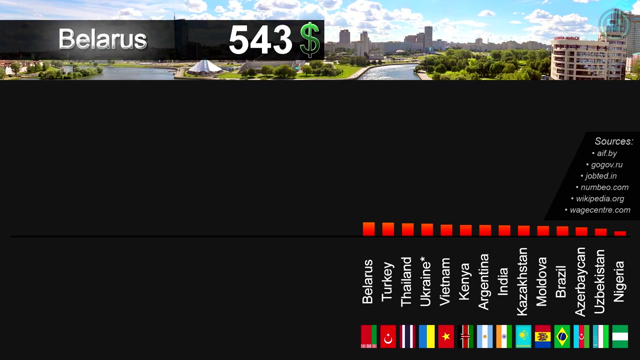 It is very important for us, the Turkish people, to open the door of participation here. It is very important for us, the Turkish people, to open the door of participation here. Calm down, gentlemen. Even if the whole world is against Lukashenko today, he will still become the President if he wants to. 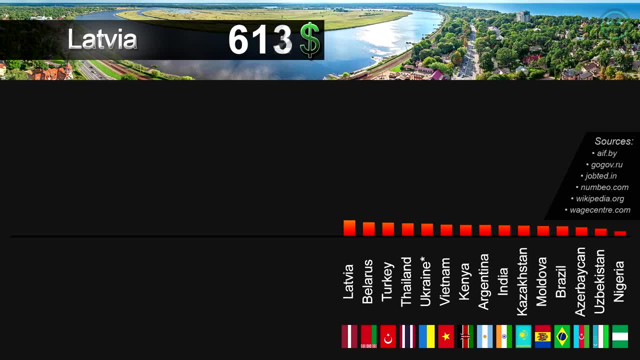 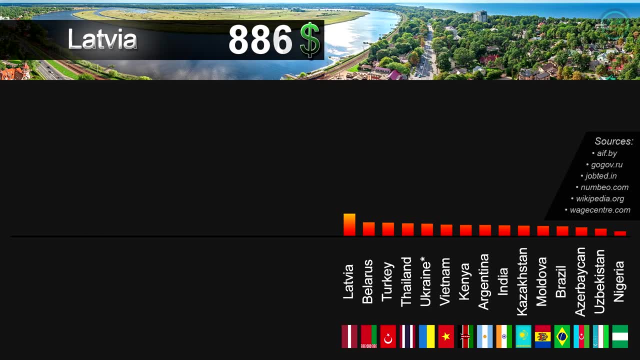 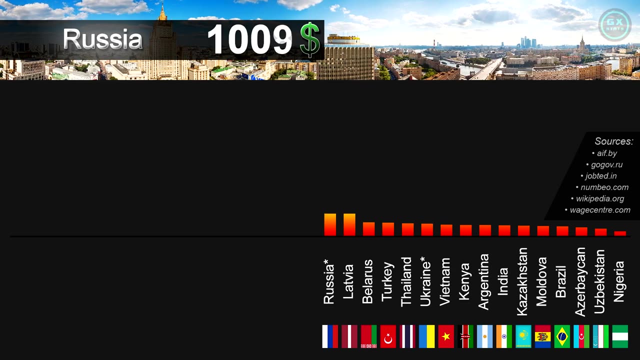 The old tradition of our people is to unite the forces in the right time. Calm down, gentlemen. Even if the whole world is against Lukashenko today, he will still become the President if he wants to. Everyone should know that we are real patriots of Russia. 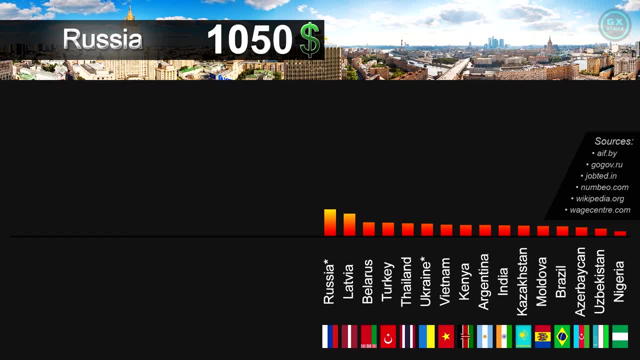 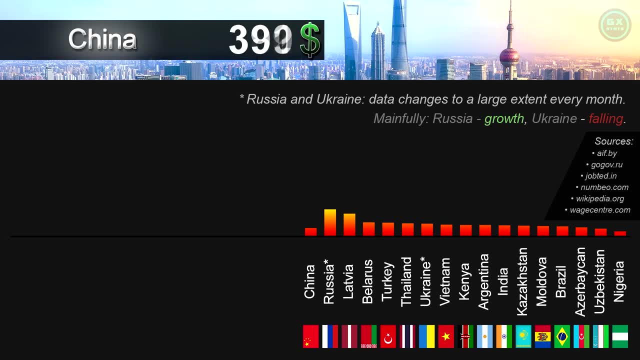 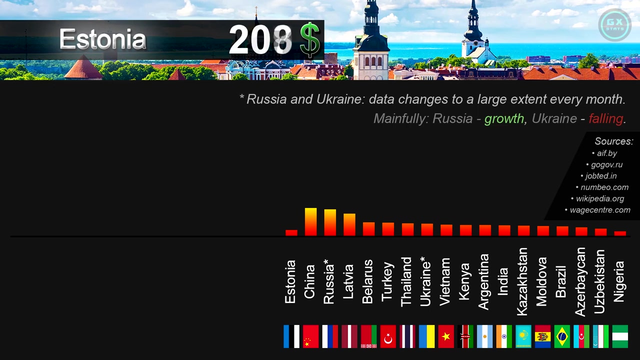 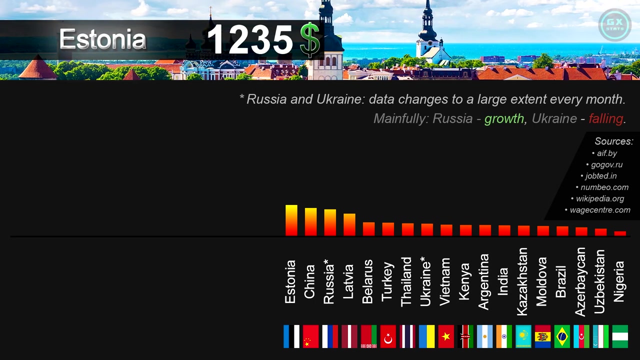 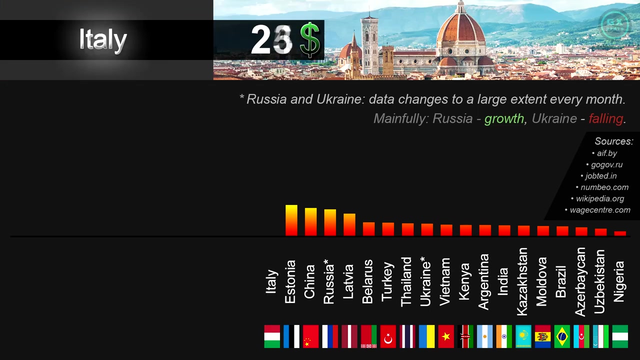 We haven't started anything seriously yet. Long live the great and glorious Chinese Communist Party. Long live the great and glorious Chinese Communist Party. The COVID-19 crisis has put digital technologies higher in our agendas than ever before. Ladies and gentlemen, we must all be brave. 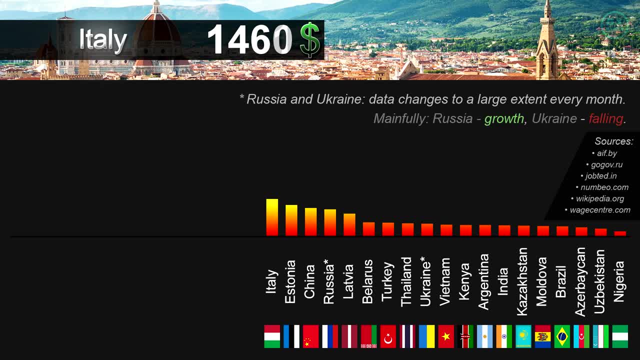 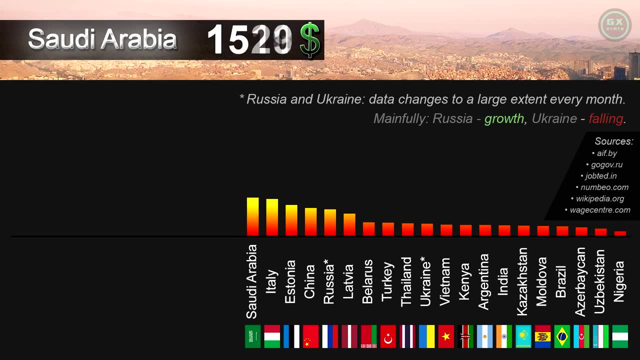 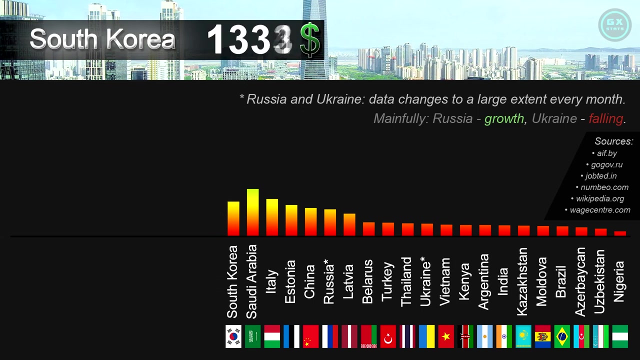 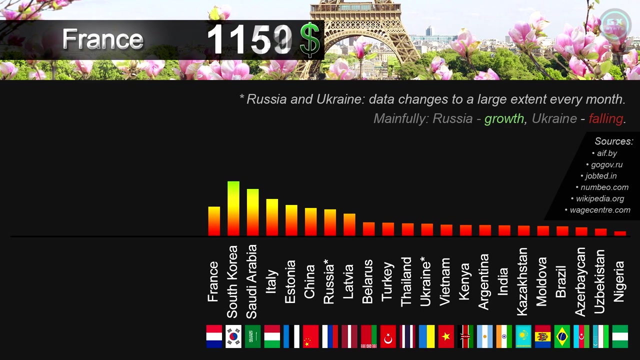 You are not going anywhere. That's mine. This is a Hands Off. This is the best. The prosecutor is not the only judge. Hey, you listen to me. Hello, thank you very much. my friends, my friends, Faced with this, I know the energy of the French people. 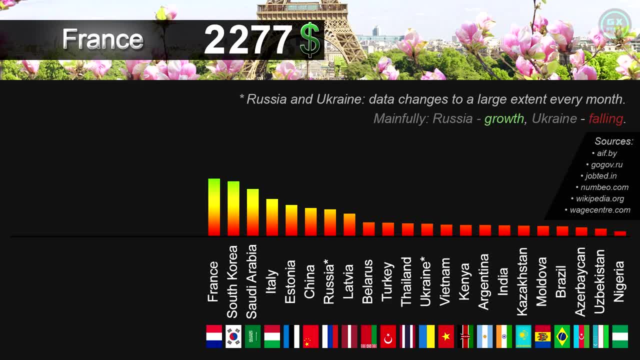 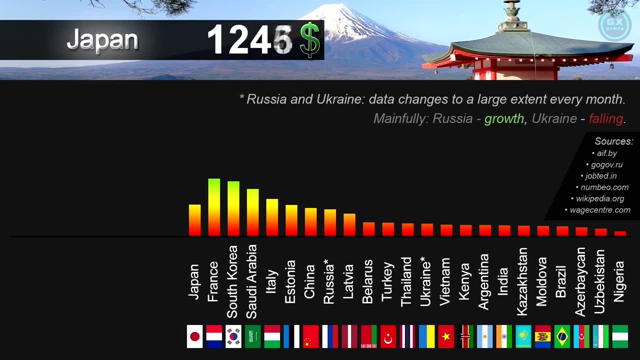 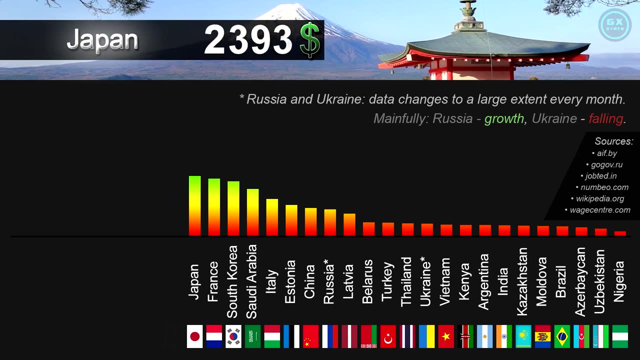 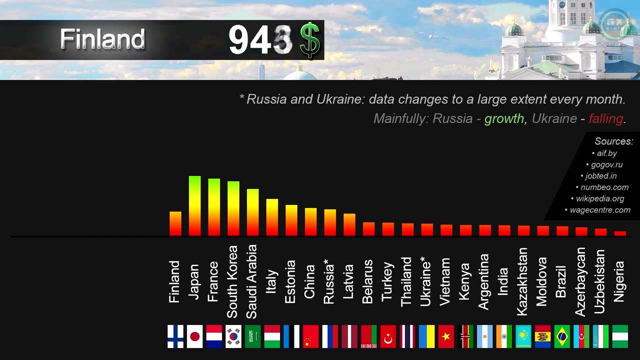 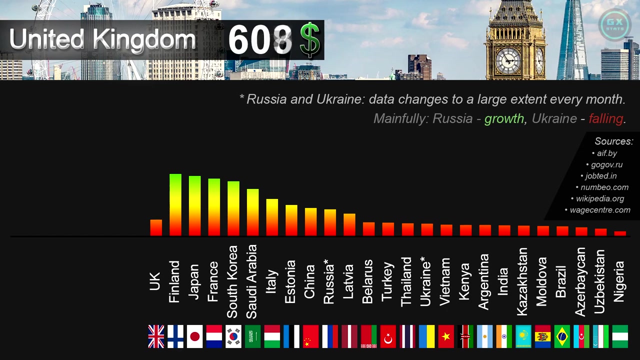 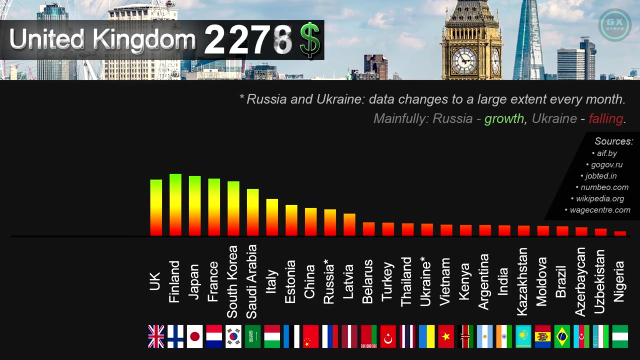 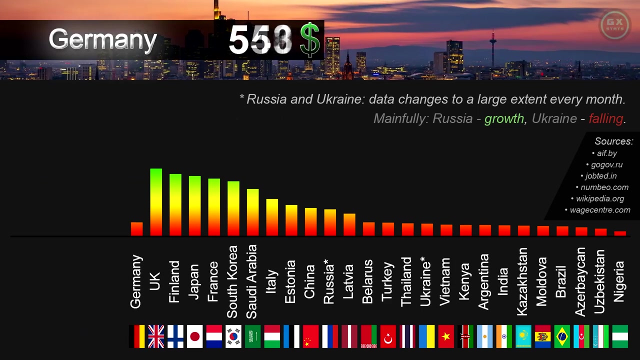 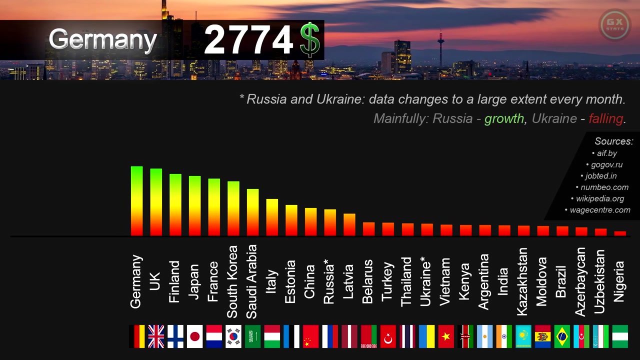 It can lead us to give the best of ourselves. I say to all the doubters: dude, we are going to energize the country, We're going to get Brexit done. I'm fat, Can you hear me now? An attentive person and not someone who only says agree. 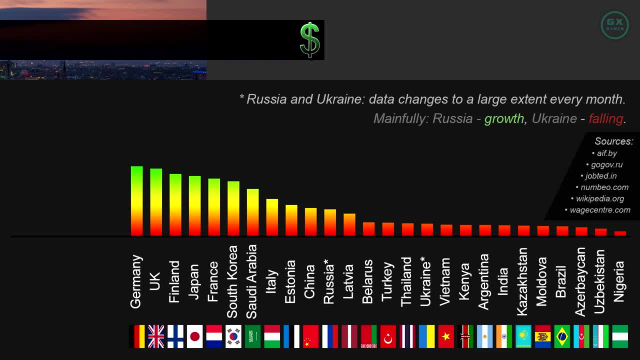 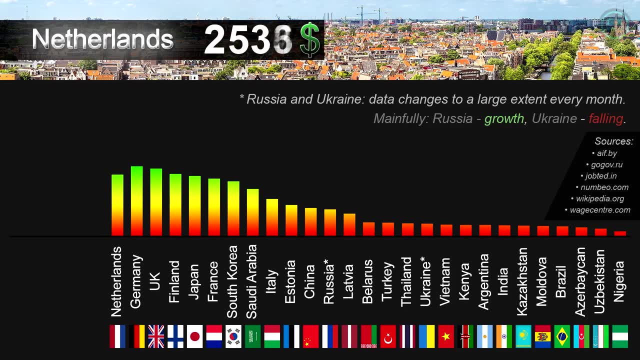 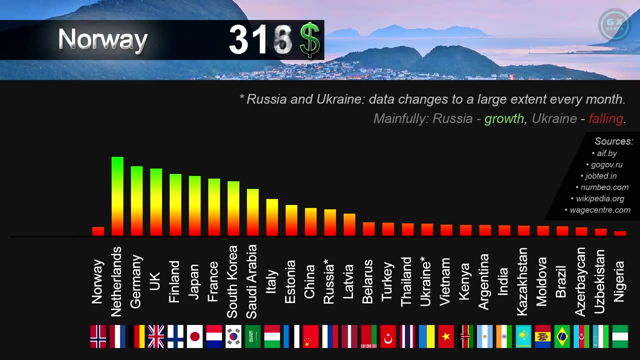 Okay, If you want future global development, you have to change. We need smarter, more sustainable and circular economies, better public, private and non-profit developments. I don't know what you're talking about. Of course it's in the first place. 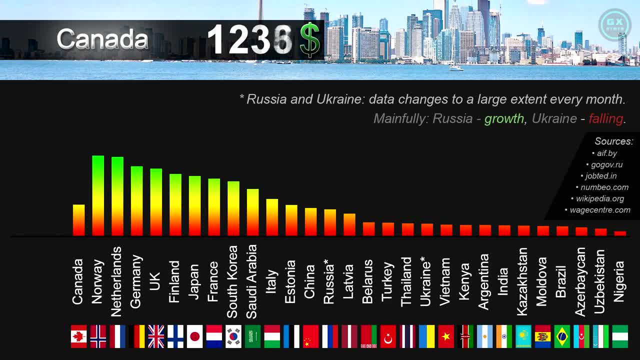 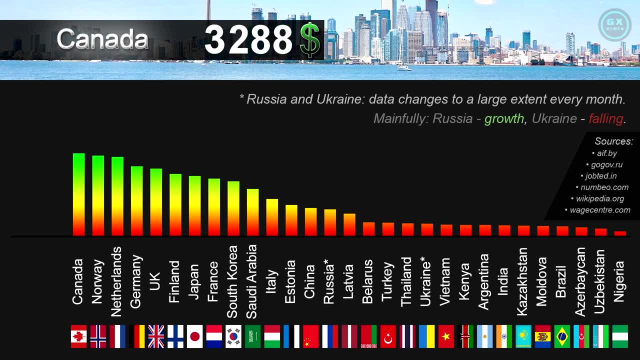 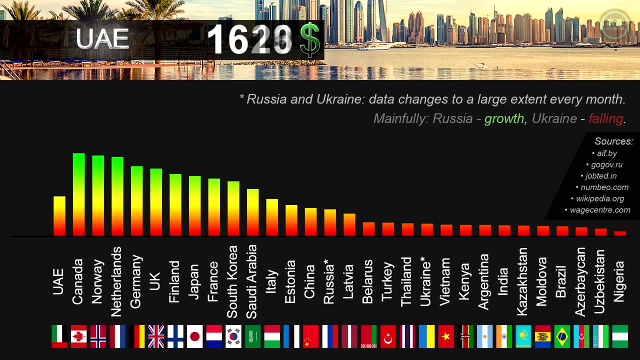 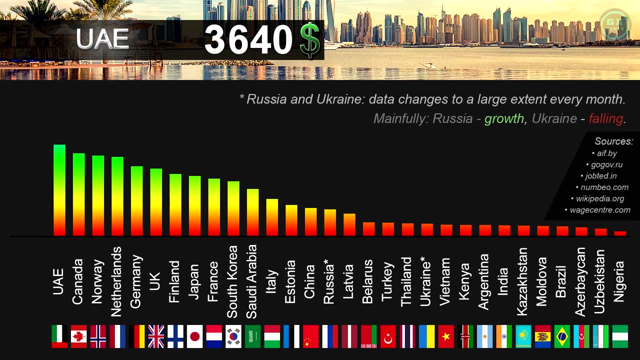 Let's ask ourselves the question: If France fails to ratify a free trade agreement with Canada, with which country do you think it will be able to do so? Thank you very much. We are not perfect and we try to change Any mistake, anything we go in and try to change. 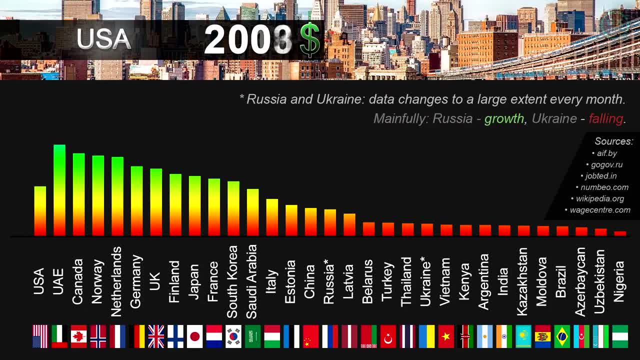 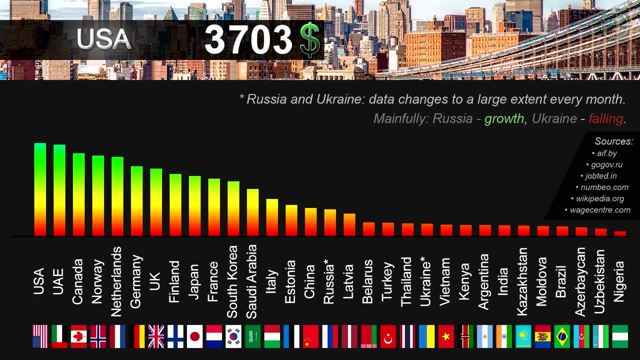 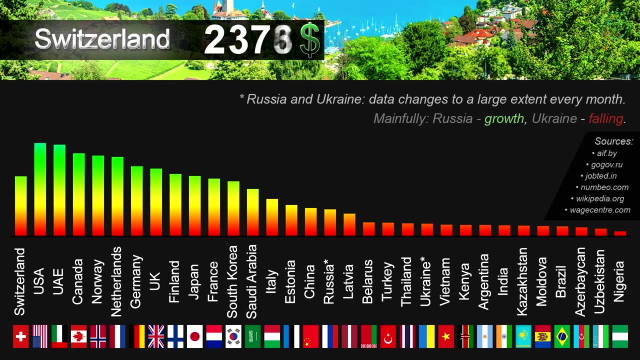 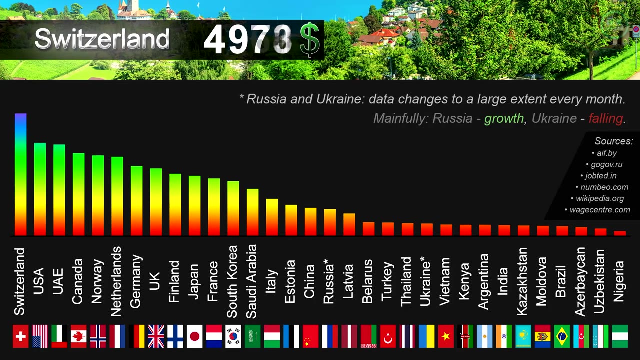 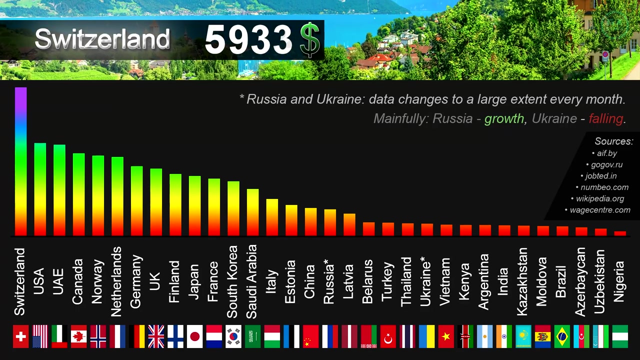 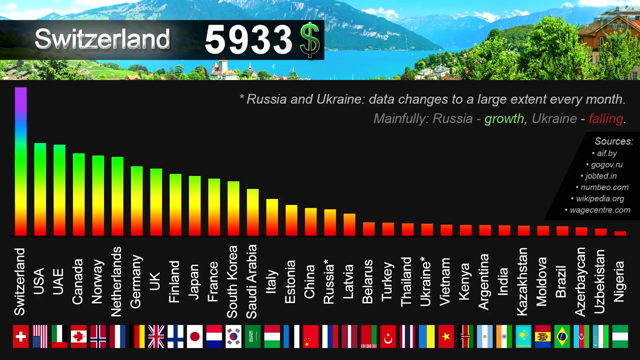 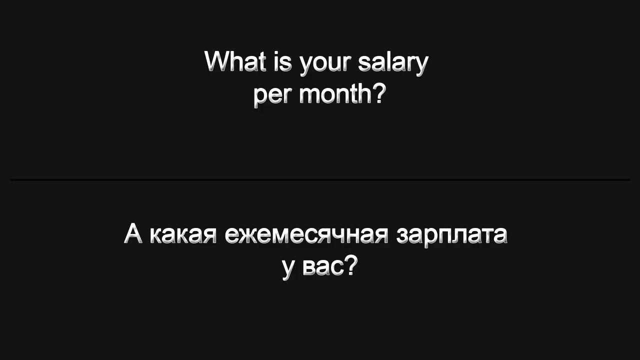 From the time I got to the Senate 180 years ago. Faced with a global challenge, our answer must be clear and clear. I warmly invite you to actively participate in the creation of a world of tomorrow. Thank you for your attention. Join us. 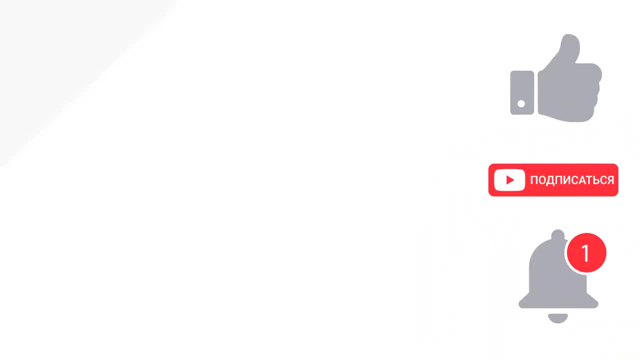 Learn more at wwwnasagov NASA Jet Propulsion Laboratory, California Institute of Technology.